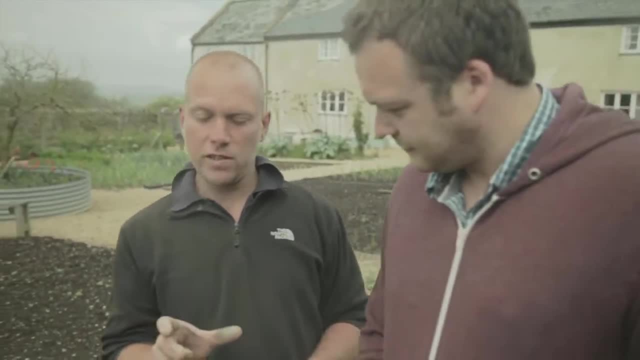 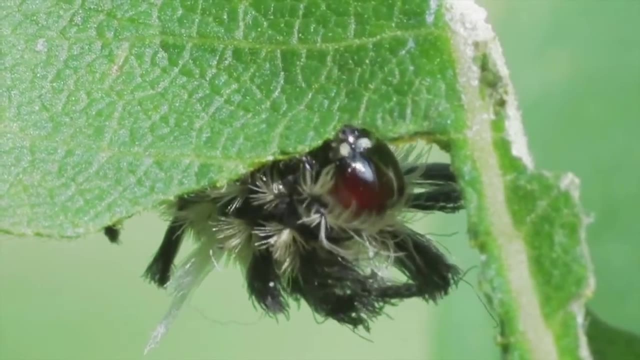 child was garden tiger caterpillars, these big furry things that used to see marching across pavements and patios. They've all but disappeared in the south here, and it's believed to be due to climate. The overwintering larvae have been rotting off, been attacked by 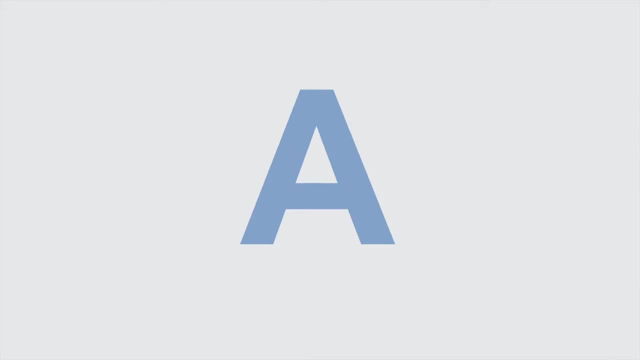 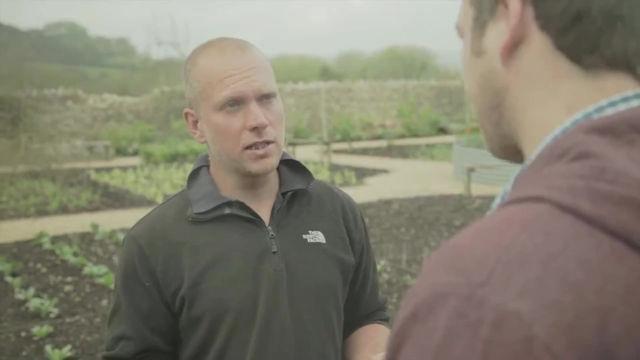 funguses, and so they're actually moving further north. Have you got a question you'd like us to take back to the Metaverse and get some answers around climate change? for Absolutely, I'm a keen ecologist, obviously, but also a keen amateur beekeeper, and with our bees being under attack, 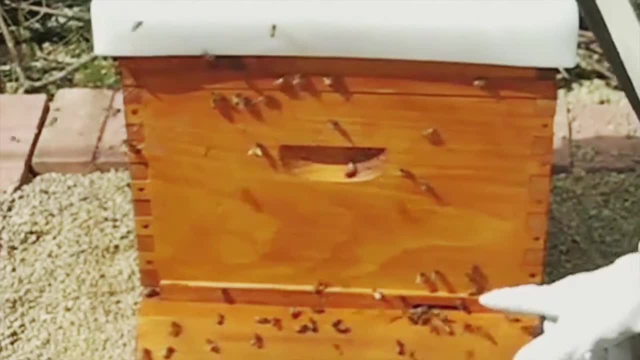 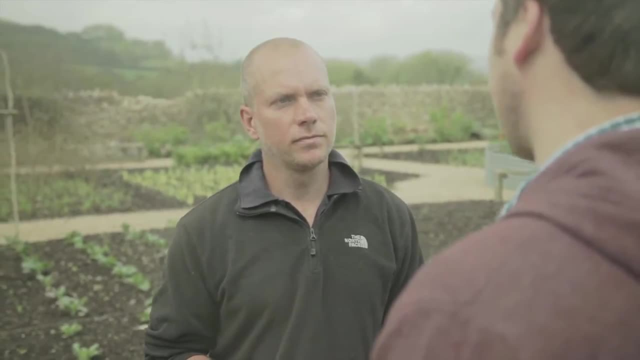 from neonicotinoid pesticides and various other things like varroa mite. I'd just like to know how our insects are going to survive in the future with the changing climate. Well, that's a great question. What we'll do is we'll take that back to the Metaverse and we'll take that back to the. 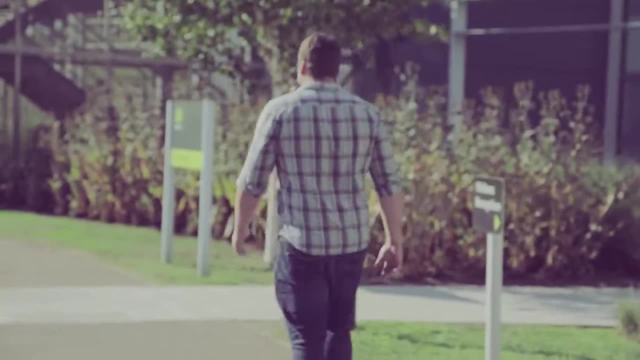 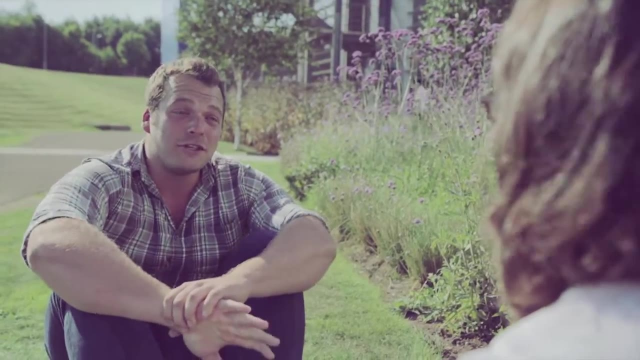 Metaverse and see if we get some answers. That'd be great. thanks very much, Hi, Debbie. thanks for joining us here. and so, as you know, recently we were speaking to Craig, the head gardener at River Cottage and obviously a massive connection, personal connection, to 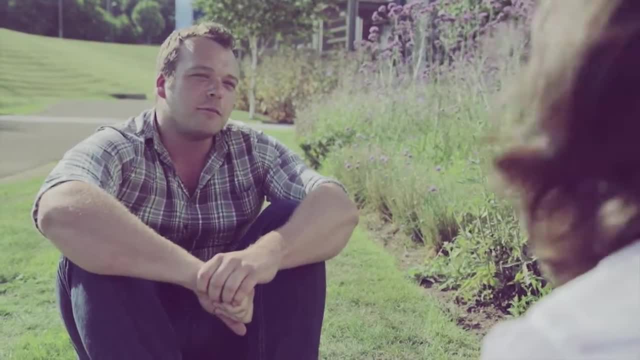 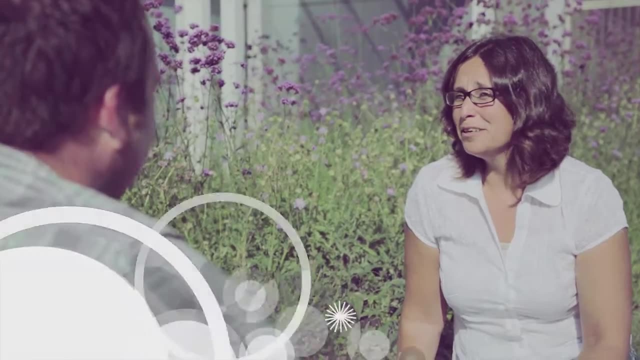 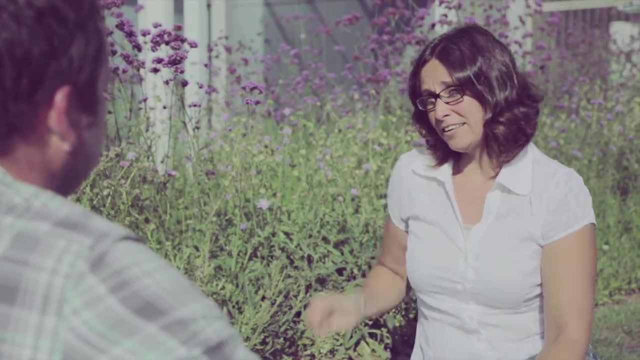 to the environment, but a particular interest in insects. So perhaps you could start off by telling us: what sort of relationships do we have to insects on our planet? Insects are vital to the planet and to our survival. really, There's about a million different species of insects globally, which is the largest group of 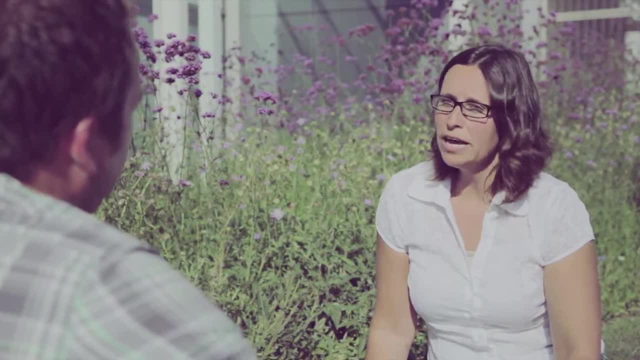 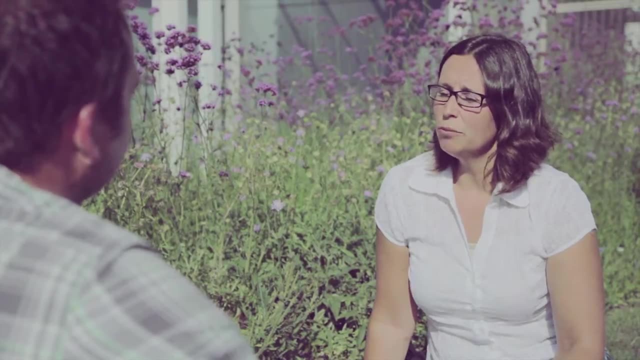 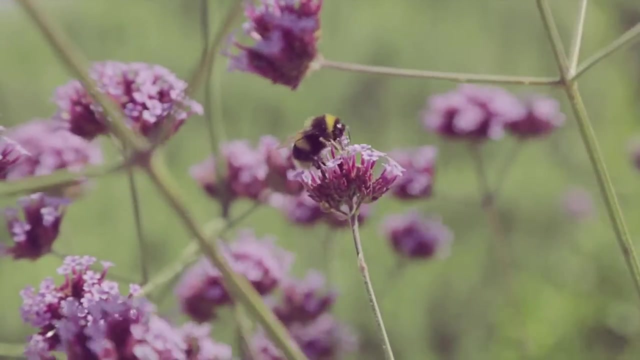 animals on the globe and about 24,000 different species in the UK alone. Insects provide a vital service to the environment. The pollinating species, for example, of which bees are an obvious one, pollinate about a third of the food that we eat. Debbie, we see them every day, but how much do? 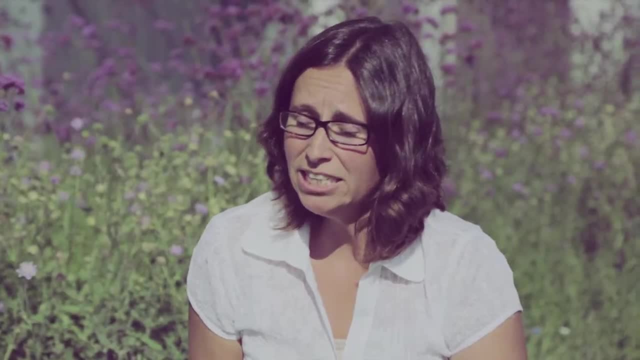 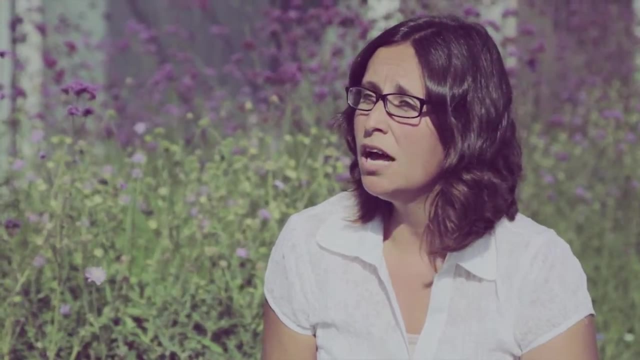 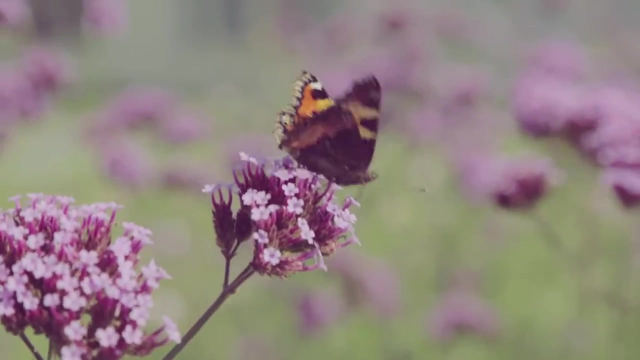 we actually know about insects. We're very lucky in the UK, actually, that we've got some of the longest records for observing certain species of insects in the world. Some of these, for example, is the butterfly survey, which is run by the Centre for Ecology and Hydrology, and butterfly.